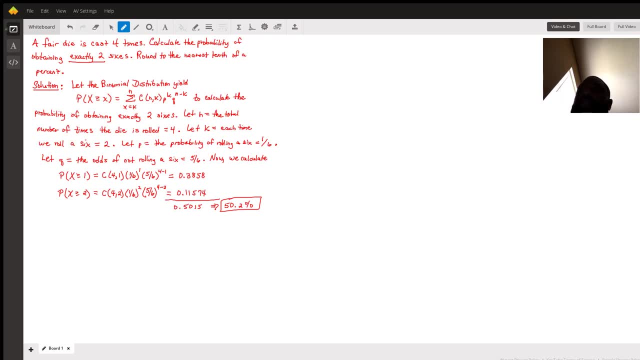 Let N be the total number of times the die four times The die is rolled, which is four. Let K represent each time we roll a six, which is two, And let P be the probability of rolling a six, which is one over six. 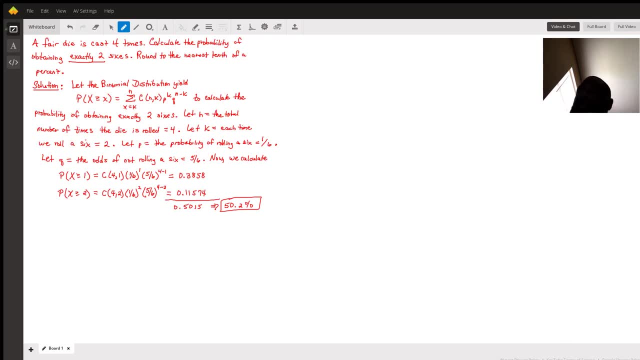 And let Q be the odds of not rolling a six 5 over 6.. Or instead of odds you could say the probability of not rolling a six 5 over 6.. Now we calculate the probability. First we got to calculate the probability after rolling a six one out. 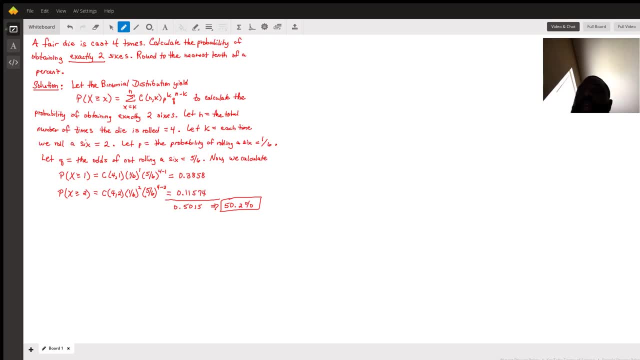 of four times when k equals one. So combination of four comma one times one over six to the one, power times five over six to the four, minus one exponent came out to be approximately zero point three, eight, five, eight. Now we have to calculate the probability of rolling. 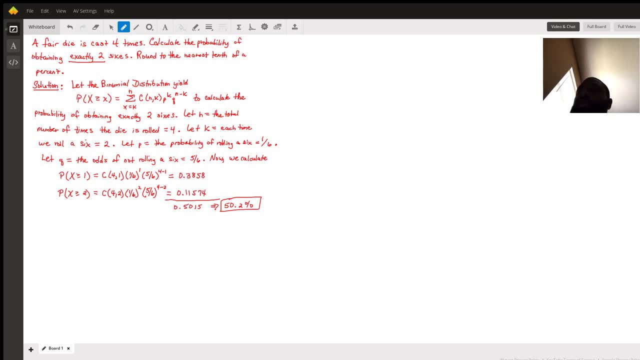 a six, a second time out of four. Combination c of four comma, two times one over six, squared times five over six to the four minus two exponent, That is approximately zero point one, one, five, seven, four. The last step is we add the two decimals together to get zero. 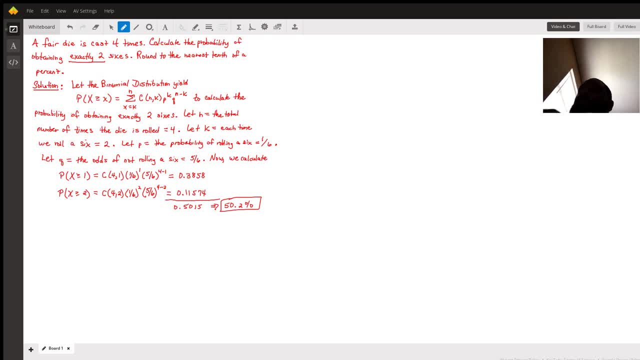 point five zero one five. Then we multiply that decimal by one hundred to convert it to a percent. Fifty point one five. Then we round it to the nearest tenth, as required. Fifty point two percent. Okay, What you notice is very much accurate, because out of four, 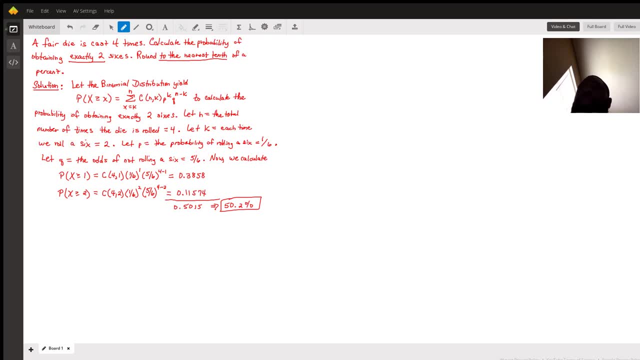 times the probability of obtaining exactly two sixes means we rolled two sixes out of the four times we rolled the dot. You see that I hope this helped. My name is Tim, Thank you.